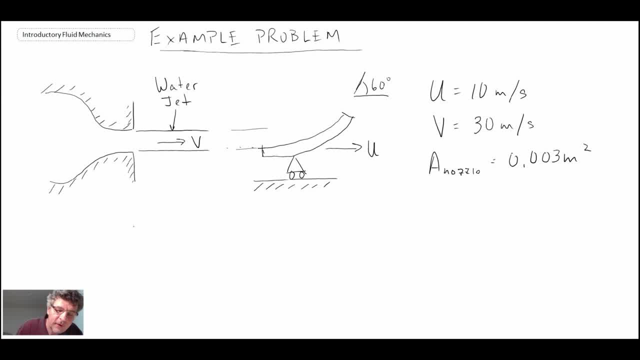 And so what we are told to solve for in this problem, we're told to find the force, So we're told to find the force on the vane in order to keep u constant. So, essentially, what we're told to do is we're told to find the force on the vane in order to keep u constant. 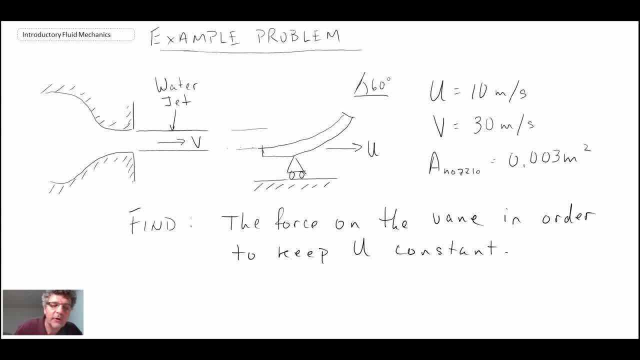 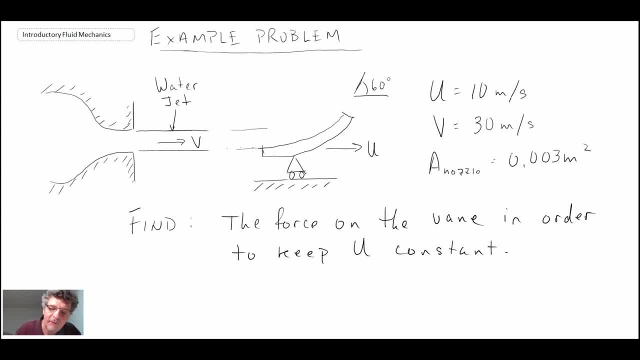 So, essentially, what we're told to do is we're told to find the force on the vane in order to keep u constant. told is: what is the force required on the vein? so this is our vein. here there will have to be some force, and we don't know exactly which direction it's going to be moving in, but a 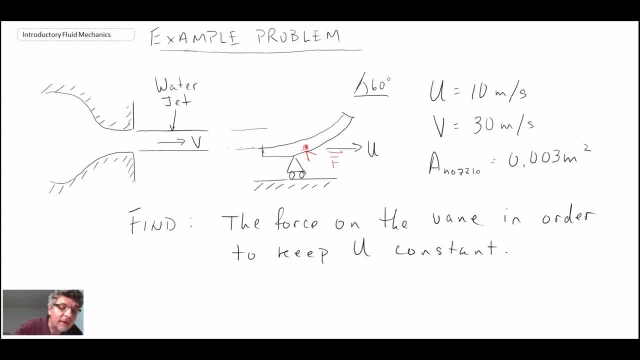 force, something like that. let me clean it up a little bit: that's not the nicest vector, but we have some force that we're looking for and the purpose is to find for u to be constant and consequently, that would be a case of a control volume moving a constant velocity, because 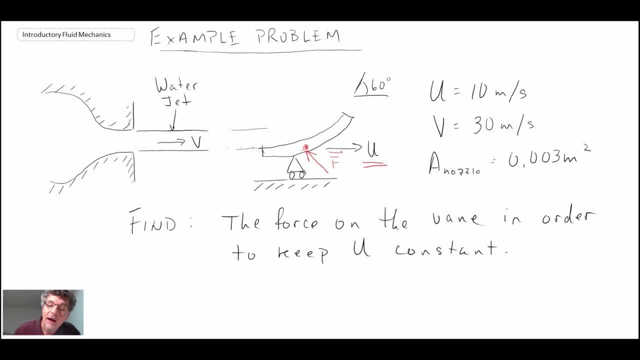 you can probably figure out, we're going to put the control volume around the vein- things that are given. we're told that the velocity of the cart to begin with is 10 meters per second, and that's the velocity that we want to maintain, and the jet is coming in at a higher velocity. it's. 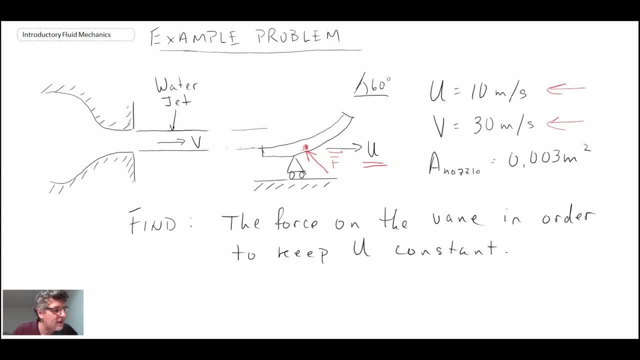 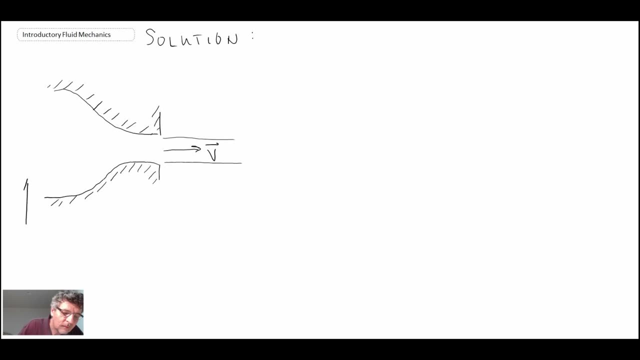 coming in at 30 meters per second. so this is a case where we will be doing analysis using a control volume moving a constant velocity. so let's take a look at the solution. okay, so what we have here? this is what our problem looks like we have the cart is moving at velocity. 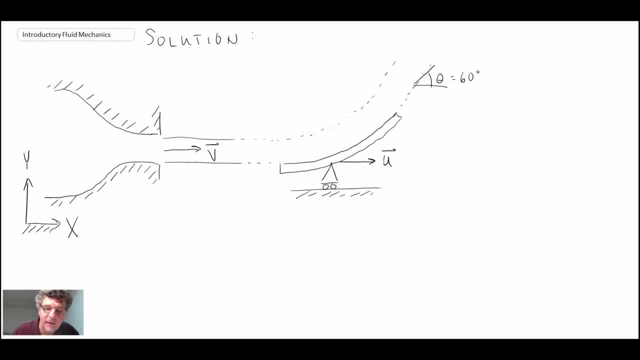 U and I'll draw that as a vector going in that direction. the jet is coming in from the left. now, what we're going to do, we need to specify the control volume and for this problem, what we're going to want to do is have the fluid crossing the control volume perpendicular to the control. 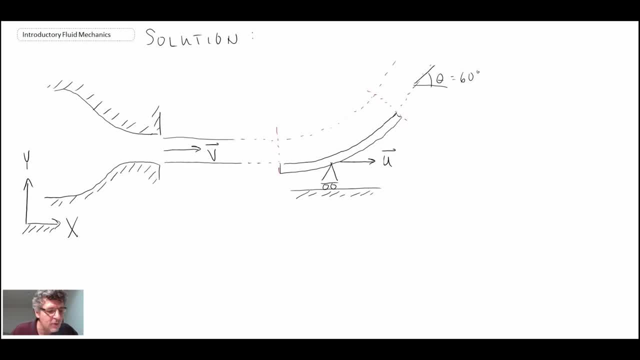 volume itself. so we will draw the control volume like that, so that it is perpendicular to the fluid streams, and then I'll come over here, the control volume, I'll bring it right down to the ground- but it's not going to go to the ground exactly- and then I will bring it up. so this is 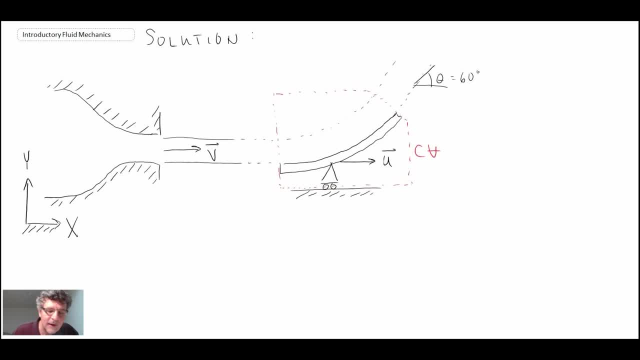 control volume that we will define, And what I'm going to do, given that we have fluid crossing this boundary and this boundary, I'm going to call this control surface one, and this will be control surface two. And then the last thing. well, another thing that we'll do, remember. 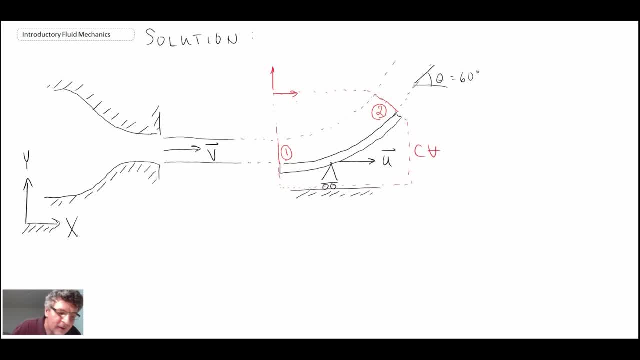 this is a control volume that is moving, And so it's moving. we have a moving reference frame. we'll give that a little x and a little y And what we're going to do, just so that you can picture what's going on. we're going to draw a little person on here, because that person is 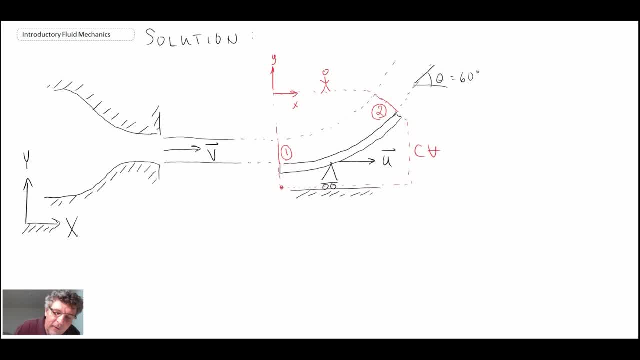 moving with the control volume. And then, finally, we're going to look for a force in order to maintain the velocity u at a constant value, And we will have a reaction force in the y direction and a reaction force in the x, And I've just drawn them in that way: positive x, positive y. 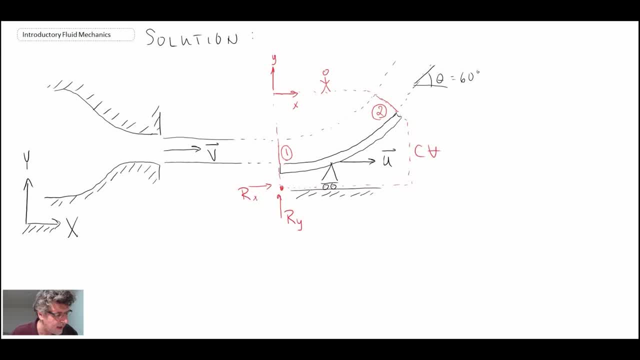 We'll have to see by the sign that we get when we're done, which is the reaction force in the y direction They actually go in, which is kind of a typical thing that you always do in statics. So we have the fluid coming in, The basic equations that we have. 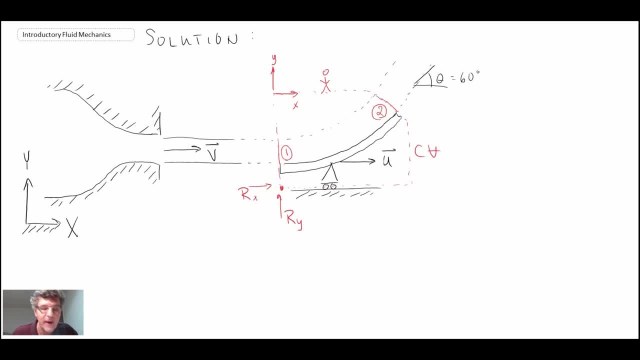 the basic equations that we'll be using will be conservation of mass, or continuity, and the momentum equation, And so those will be the two basic equations. A few assumptions. Let me write out the assumptions before we jump into the equations. Okay, so a few assumptions that we have. We have steady flow, So, even though the control volume is, 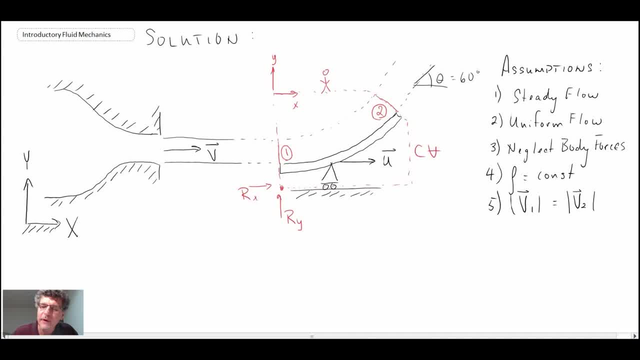 moving. it's not accelerating because the force is holding it so that it only moves at a constant velocity And the conditions coming out of the jet itself? from here we're not told anything is changing there. So as far as we're concerned we can assume that to be steady flow coming in. 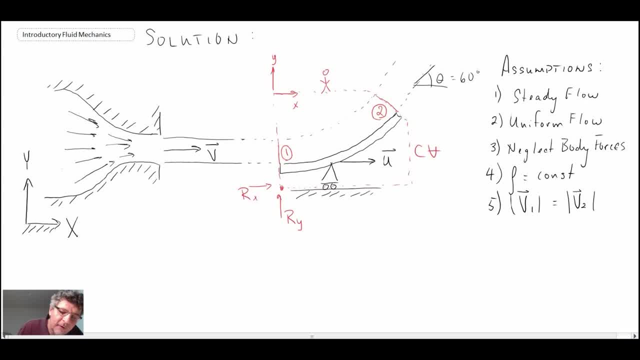 Uniform flow. So what does that mean? What that means is that we're going to assume that this is kind of a fixed velocity profile. If you were to look at the velocity profile coming in, it is uniform. It's not a velocity profile that would have some sort of parabolic or different type of shape. like that We're going to. 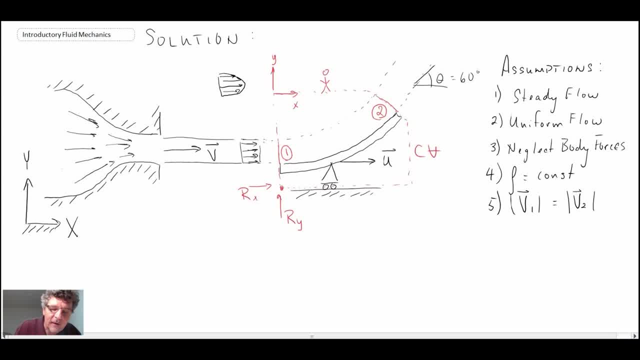 assume it to be a uniform velocity profile. Sometimes we call that the top hat profile because it would be flat, Neglect body forces. Next thing: density is constant, So incompressible flow is what we're dealing with, And the final assumption is that v1 is equal to v2.. 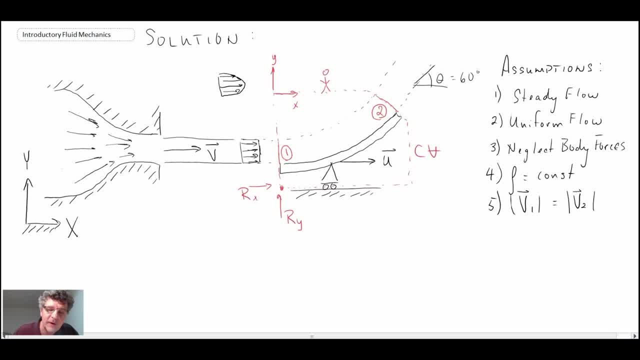 And so what that is implying? the magnitude of v1 is equal to v2.. So that would be the velocity of the fluid coming in at control surface one and the velocity or the magnitude of the velocity of fluid leaving control surface two. Okay, so those are the assumptions, What we're now going to do. 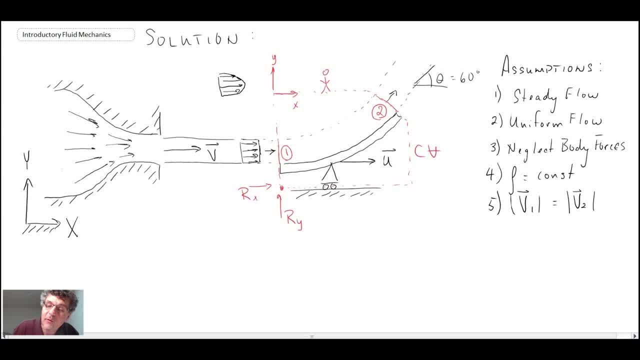 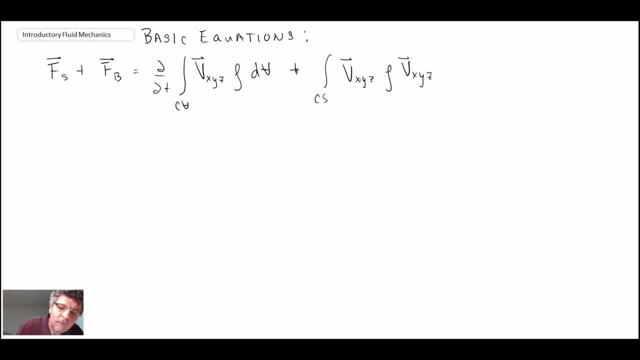 let's move ahead and start working with our basic equations. For now, what we want to do is to sketch our basic equations, start with more macro equations. Okay, so we have linear momentum And we have continuity. So those are the basic equations- continuity, The basic equations we have. let's start with. 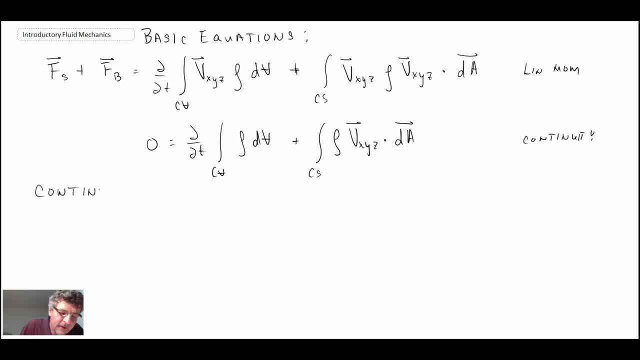 continuity and applying the assumptions that we wrote out, So we can eliminate some of the artisticmother assigns to us by trying to call this a batteryступ, Such as of the terms. so okay, so to begin with, we have steady flow. so this guy is gone and 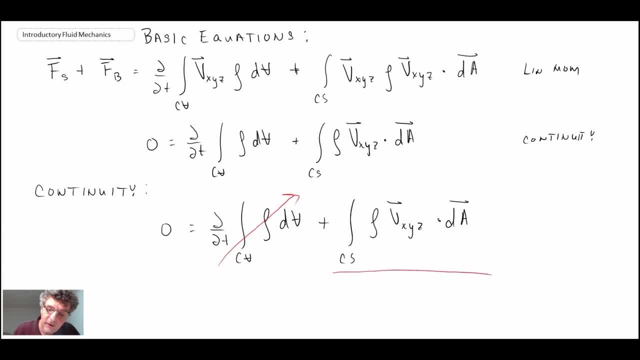 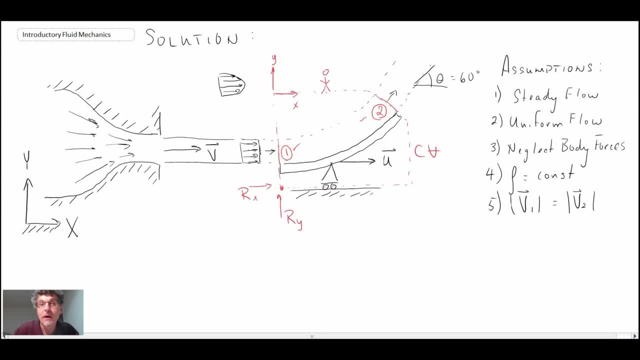 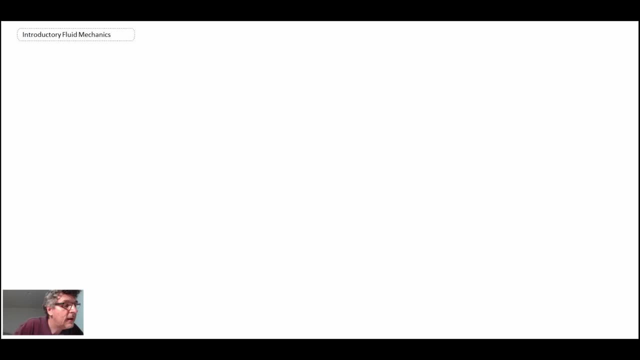 what we're left with is an integral across the two control surfaces. if we look back here, we have control surface 1 and control surface 2, so we apply the continuity equation across those two control surfaces and let's expand that out and I'm going to write the: 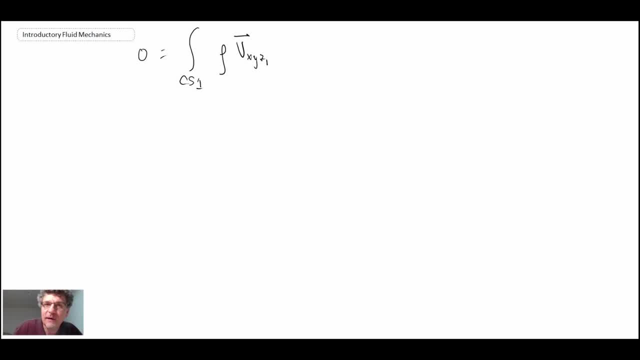 velocity vector with x, y, z. so that's in our with respect to the control volume reference frame. I'm going to put it with a little subscript 1, and then for control surface 2, we have that now writing out the velocity vector or the. yeah, that'll. 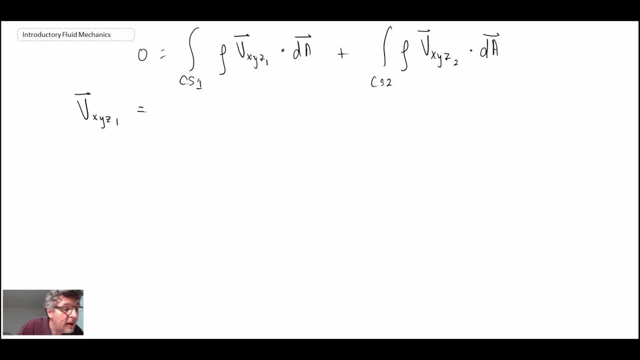 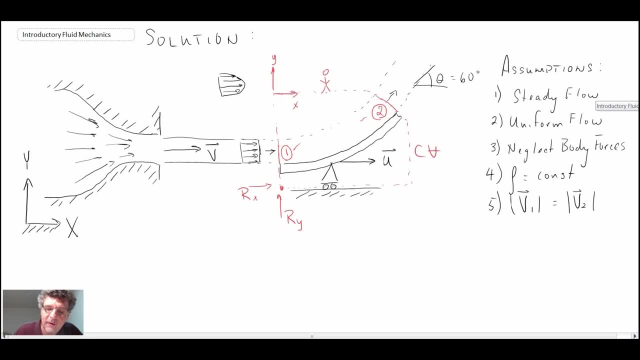 be the velocity vector at control surface 1, what we have looking back and remember. we have to. we have to deal with velocity with respect to the control volume. so we have a situation where we have v coming in and the control volume itself is moving at. 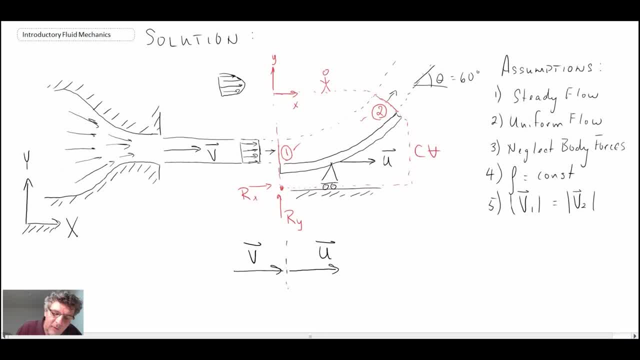 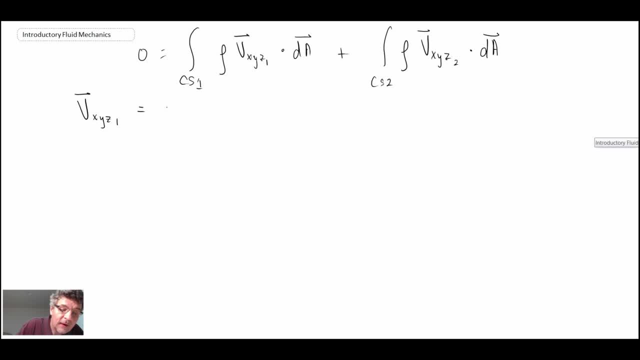 u. so the velocity coming across here with respect to the control volume is going to be the difference between those two. so we will have v minus u and then we can express that on inlet. Both components are moving in the x direction and so we get this. I can write it out in: 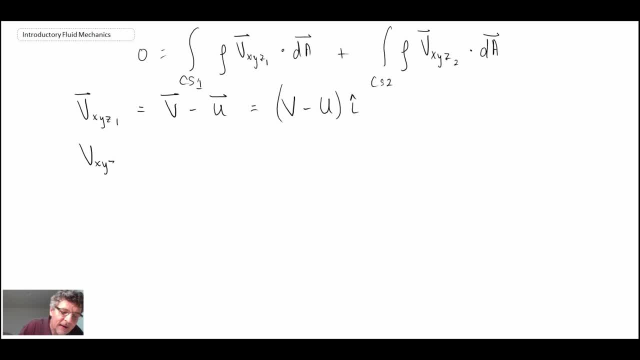 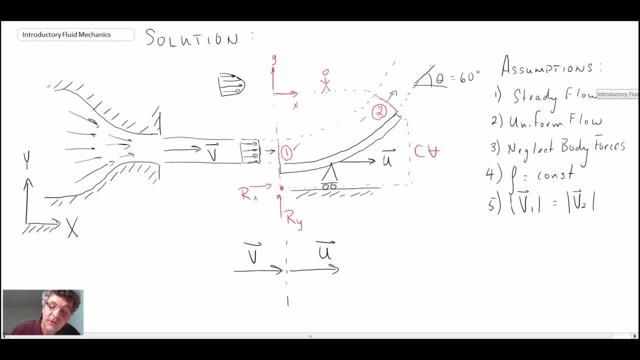 the i component and then for the velocity leaving. this is for one of the assumptions we had. we said that the magnitude of the velocities were the same. so looking back at our drawing, we know the angle here is 60 degrees, so we can use trigonometry to 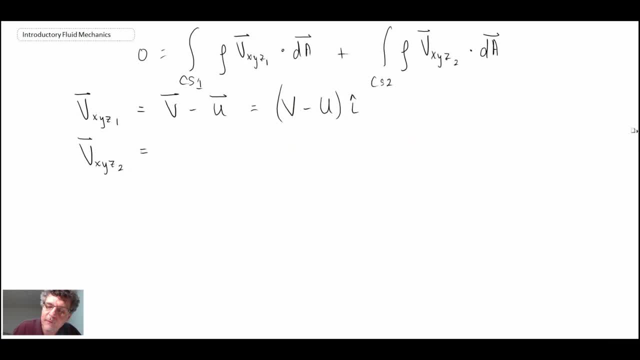 figure out what the velocity component would be leaving. Okay, So that would be the x component and the y component, and there we've made use of the fact that the magnitude of v1 is equal to the magnitude of v2, one of our assumptions. 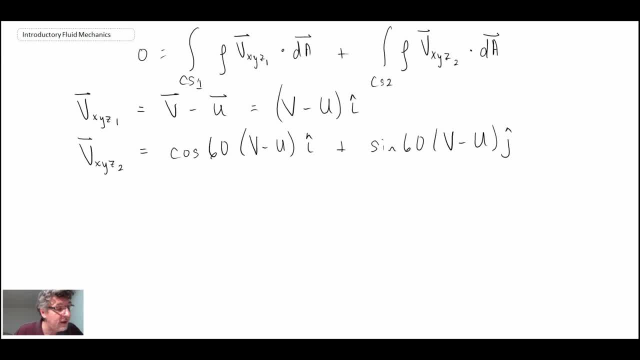 So what we can do is we can put this together And what we get for continuity and remember we need to be careful with the sign here. So for control surface 1, let me just sketch this out because this is sometimes an area.